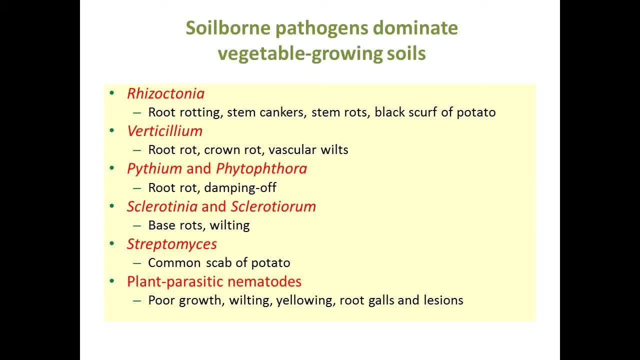 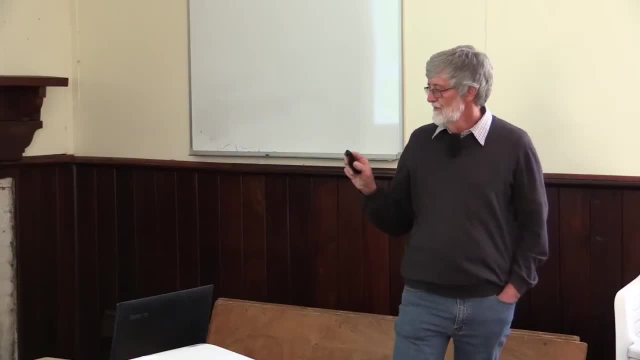 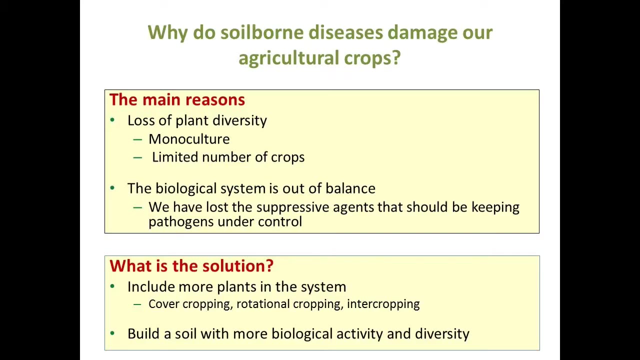 this in terms of how to deal with them, because every pathogen is different. But the main reason we have so many pathogen problems in our agricultural soils is, firstly, we've lost plant diversity, So we tend to grow a single crop or a few crops, and so we finish. 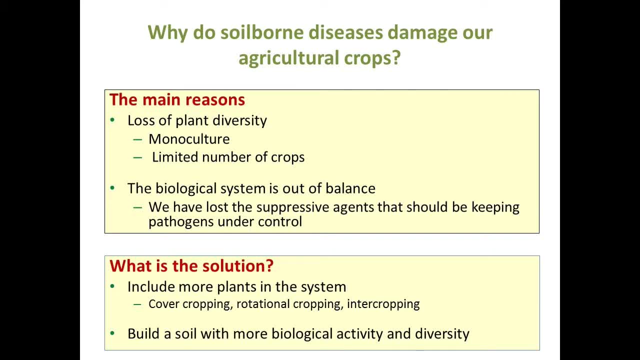 up with all the pathogens that attack those crops, And I guess what we finish up with is a biological system that's out of balance, and we've lost some of that diversity that we used to have, And so I guess the solution to that is to. 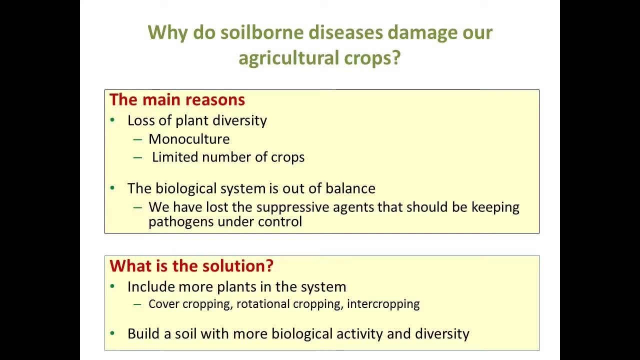 try and get rid of that diversity, And so I guess the solution to that is to try and build back some diversity by getting more plants into the system and get that diversity back. And the sort of things that can be done are cover cropping, rotational cropping And 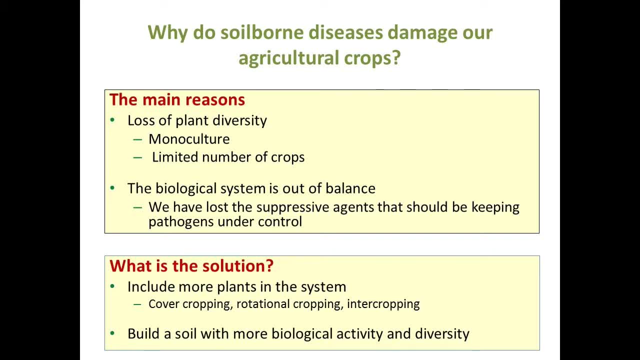 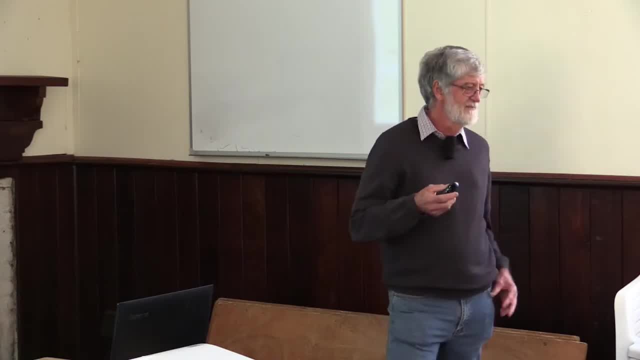 I think people are starting to wake up to this a bit, and certainly in Queensland we've got sugar growers now who, instead of growing a single rotation crop, are trying these multi-species mixes. There's a guy in Mackay who's got an H-species mix that he's putting in because 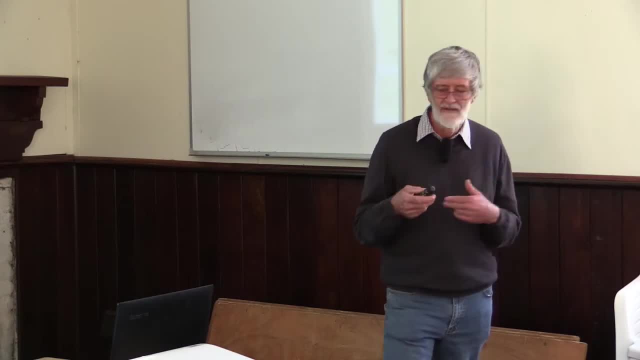 he wants to get some diversity back into the system. Now, certainly, you know we've got it's very early days in terms of you know whether we're actually getting benefits from it, but other sort of things that people are trying. So I think it's every plant is. different. You know they have different types of root systems and they, you know, some go deep in the soil, some don't. So that's all going to help in terms of creating some diversity in the system. One type of disease suppression is what we call organic matter. 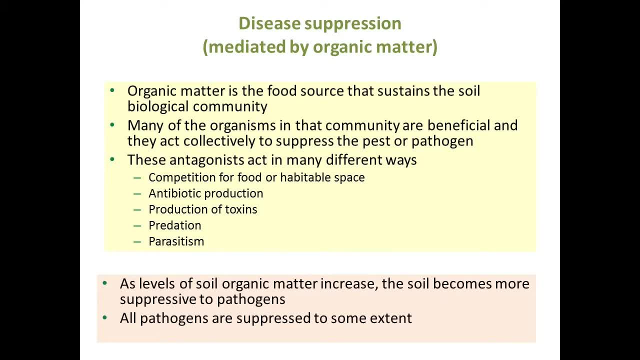 disease, mediated disease suppression. So this is where we get a whole range of different organisms that are all dependent on all the bacteria and fungi that are feeding on this organic matter And they- they collectively keep, help to keep the disease under control. 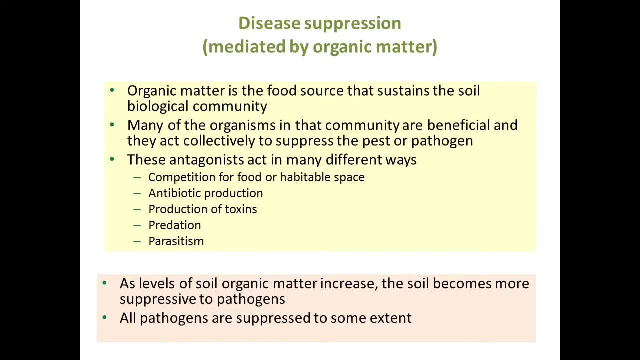 I guess they can act in a lot of different ways. They can compete with the pathogen, for, you know, for food or space They can produce antibiotics. Some, some organisms produce toxins. There's predation going on something, eating something else, or there can be parasites. 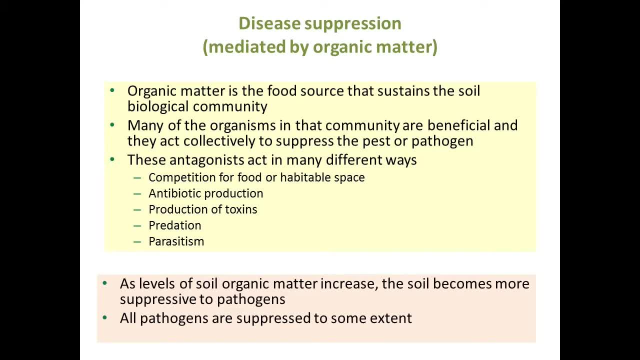 that you know parasitise other things. So I guess in general, as you increase the level of soil organic matter, you tend to get a soil that's more suppressive to pathogens. There's more active biology there and a lot more suppression And and the other good. 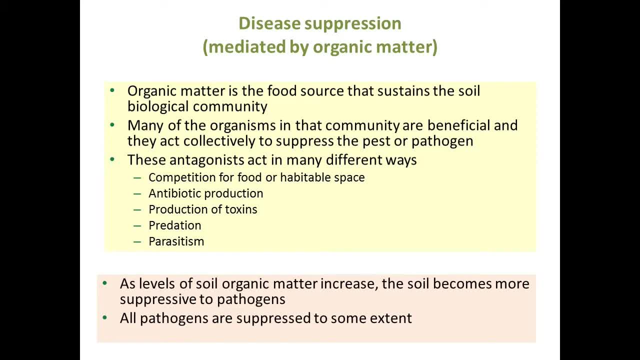 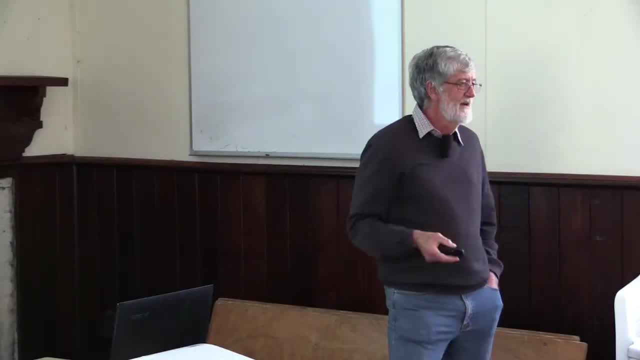 thing about it is it tends to be- it's not just a single. it usually has some effect on a range of pathogens And and so if you've got three or four major pathogens, there's a chance that there could be activity against all of them to some extent. So this is sort 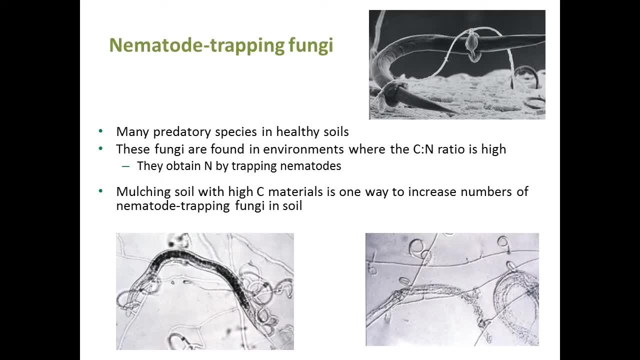 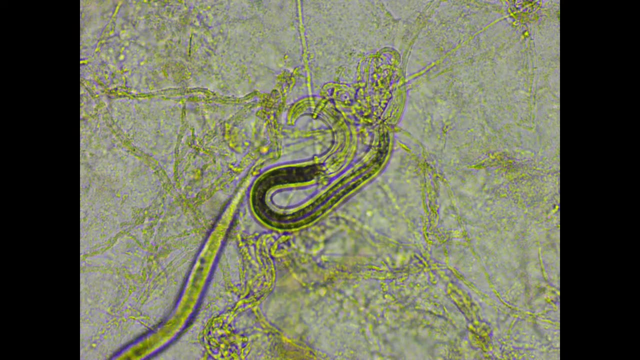 of a couple of examples. There are these fungi that that trap nematodes. They produce these traps that kill. they nematode crawls in, gets trapped by the nematode, and then the fungus then grows in and actually kills them. So that just shows a video showing a a nematode, that's you can see the trap. 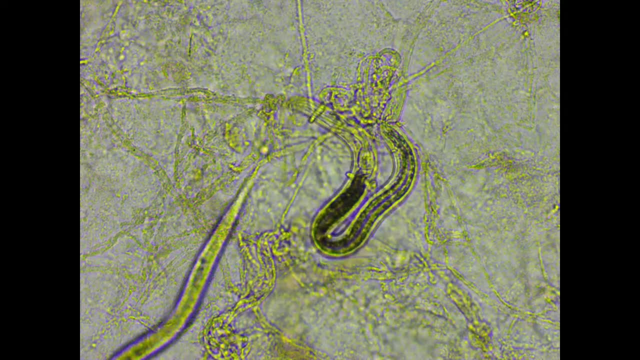 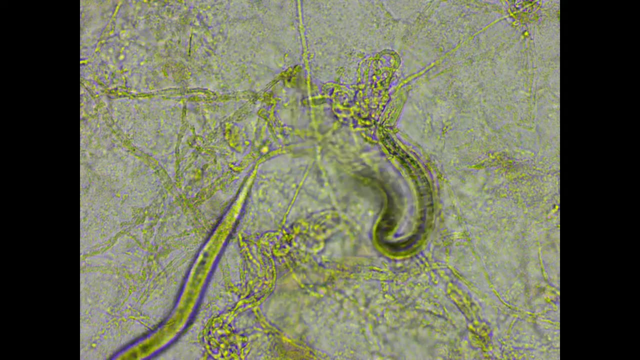 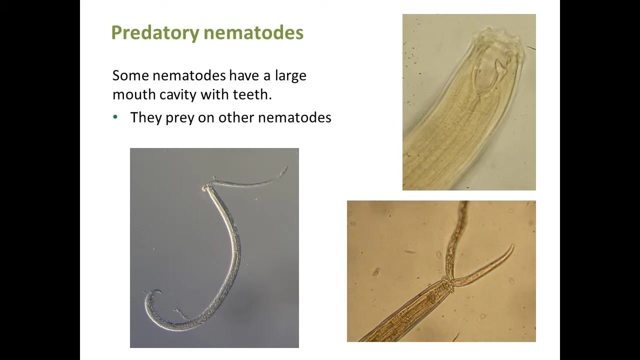 up up here. Nematodes get caught by that trap and you know a few days, probably a few hours, that nematode will be dead and parasitised. There are predatory nematodes in the soil, That's. these things eat other nematodes. 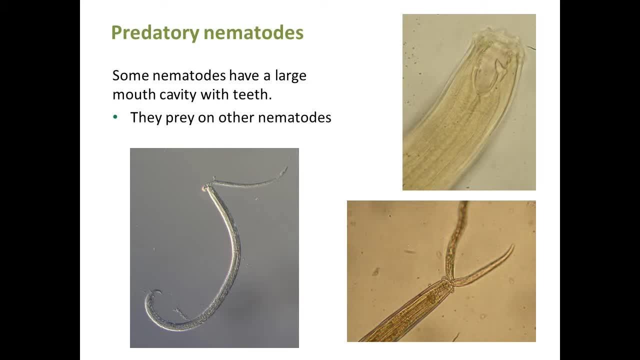 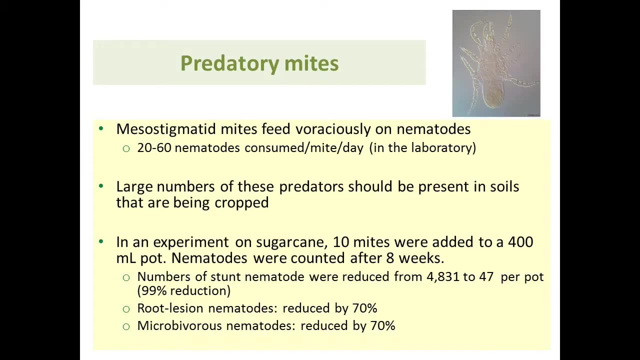 When you do a nematode sample, you want to see these things in your soil because that shows you at least got some things in there that are actually doing doing good things for you. There's also mites that eat nematodes, So these little animals are as I said about. 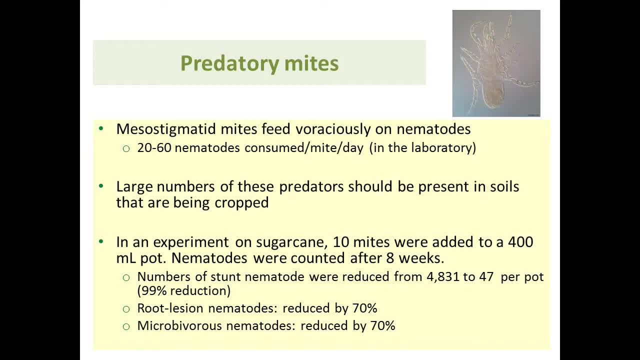 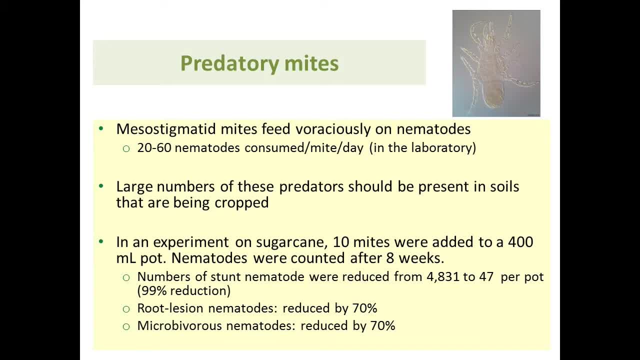 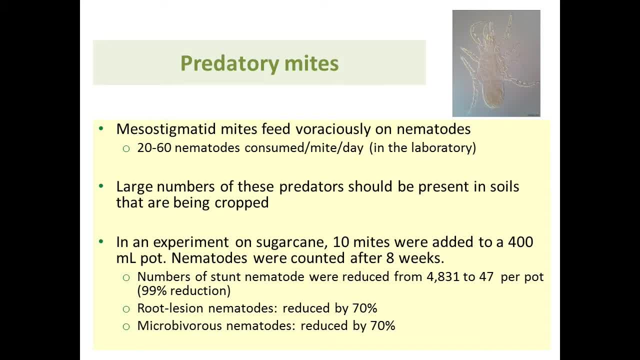 plant in it and inoculated with nematodes that attack the cane plant And I couldn't believe the results when we took it out, The this stunt nematode, which is one of the bad nematodes you know, there was nearly 5,000 in the ones without mites and only about. 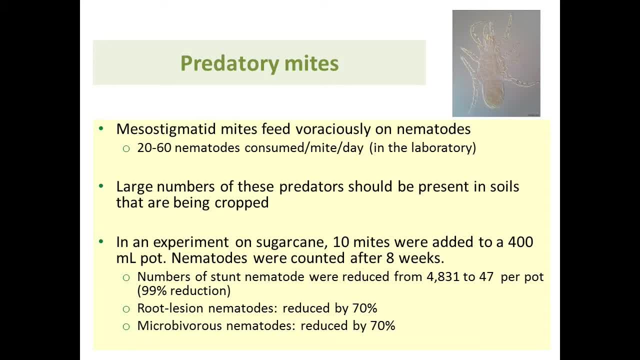 47 in the ones that had mites, so a 99% reduction. I don't usually get that sort of result with a nematocyte. That's right. It reduced root lesion nematode numbers by 70% and it also